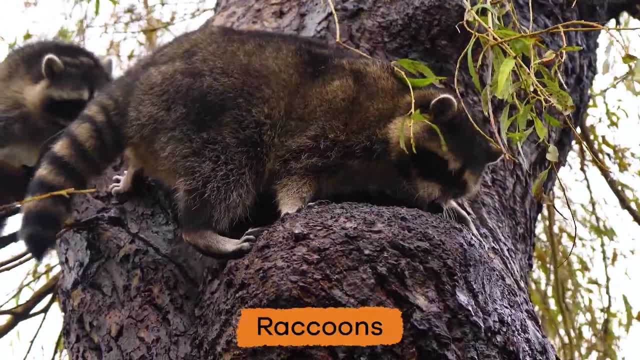 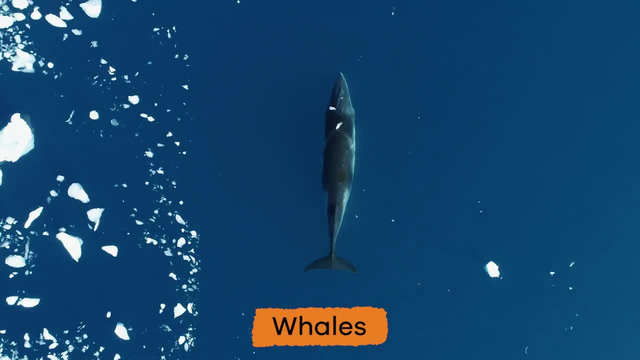 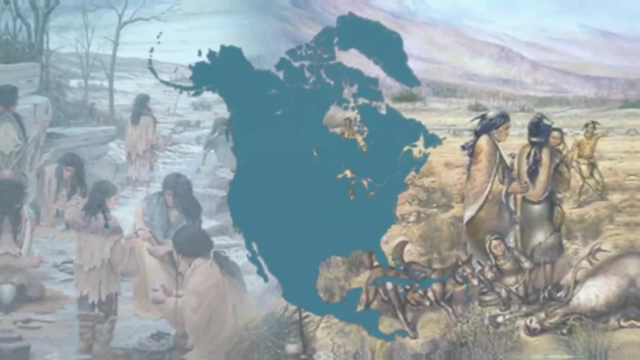 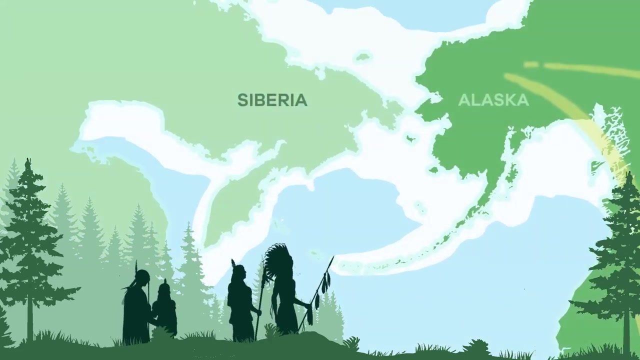 rabbits, squirrels, raccoons, deer, coyote, bears, wolves and cougars, And the continent's waters are home to whales, dolphins and sharks. The history of North America is pretty fascinating. Scientists believe that over 15,000 years ago, the Paleo-Indians from Eurasia used a land bridge. 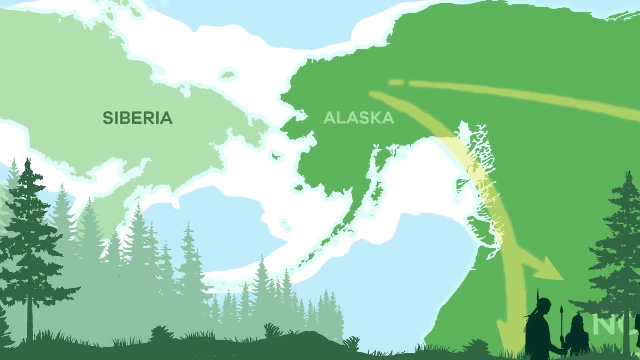 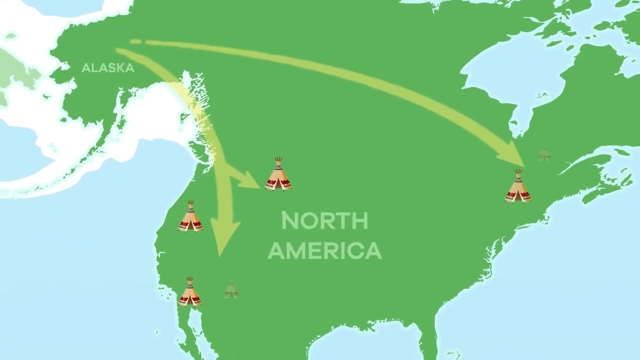 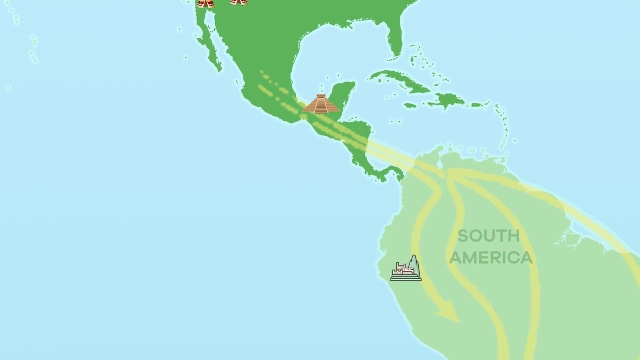 between modern-day Alaska and Siberia to travel to the North American continent and settle. The people moved south and developed organized societies and advanced farming technologies. The people moved south and developed organized societies and advanced techniques. Ancient civilizations, including the Mayans and the Aztecs, also thrived and built. 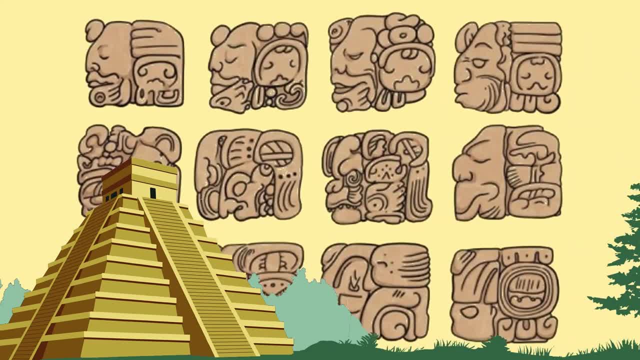 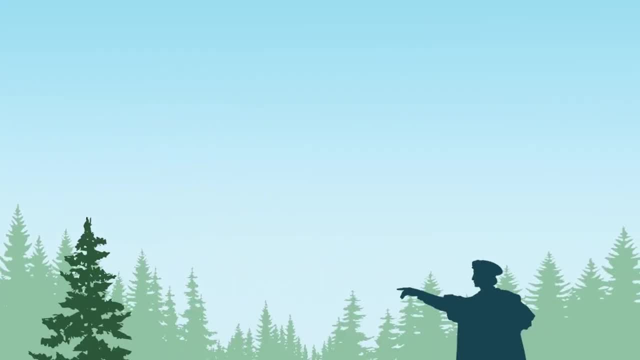 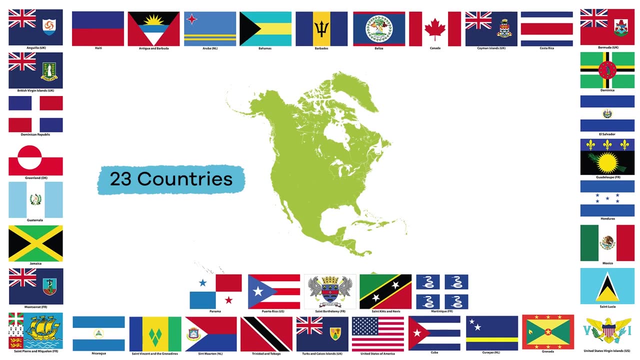 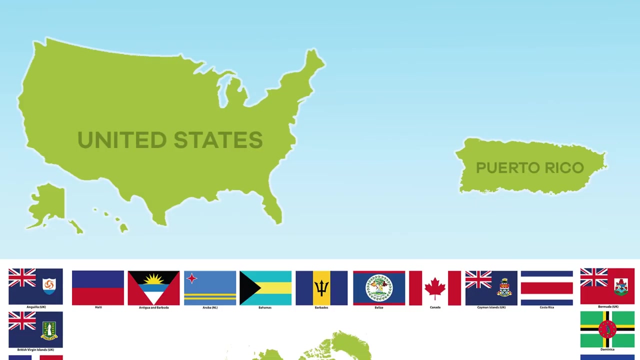 temples and created writing systems and calendars. Eventually, North settlers and colonizers from Europe also traveled to North America, often displacing indigenous peoples and settling on their lands. In all, there are 23 countries and almost two dozen dependent territories. Let's break this down. Territories are part of other countries in the world, but are still separate. 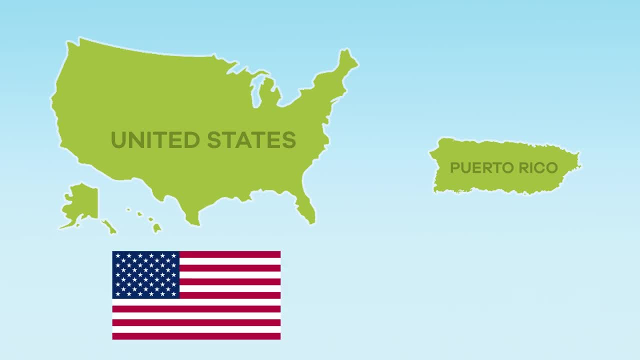 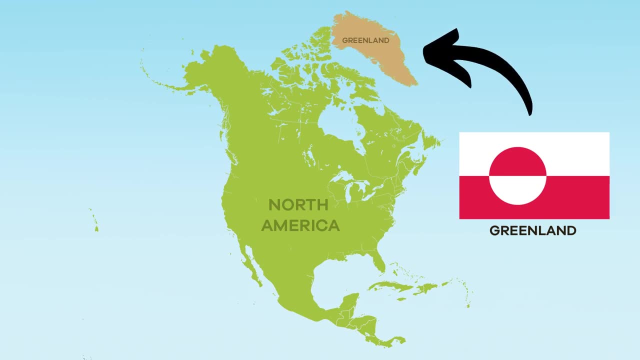 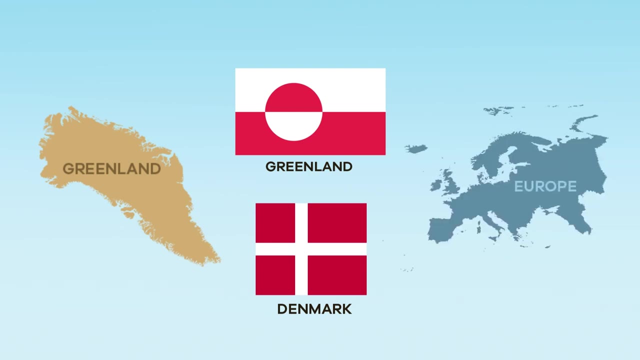 from the country. For example, the United States is a country, but one of its territories is the island of Puerto Rico, And Greenland, although it is geographically part of the North American continent, is controlled by Denmark, which is politically aligned with Europe. 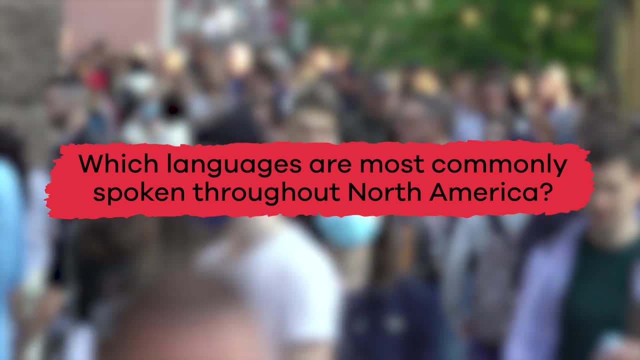 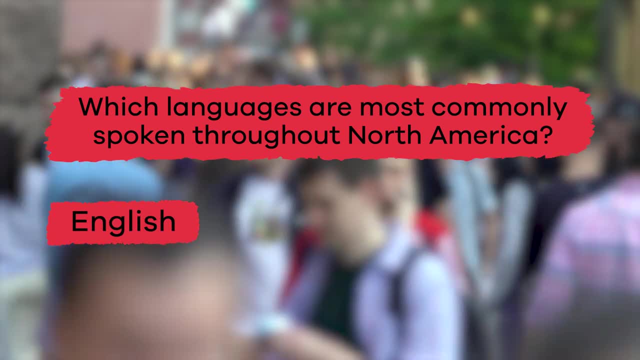 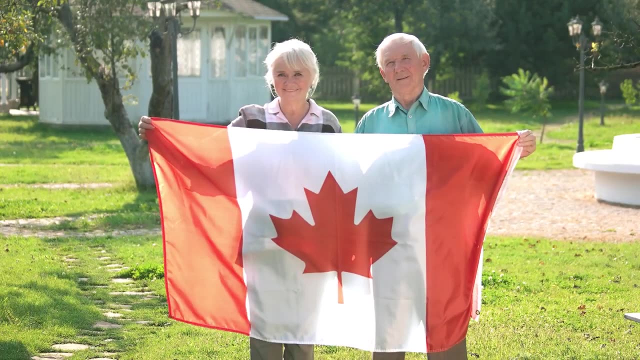 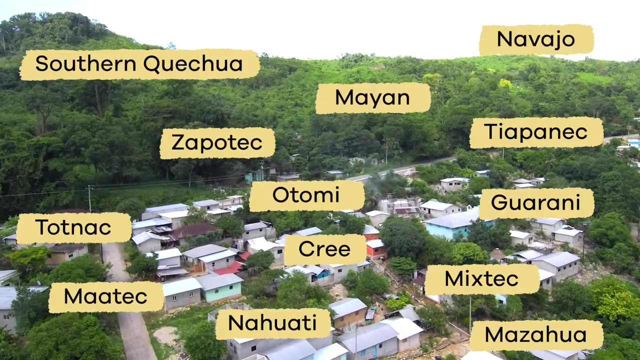 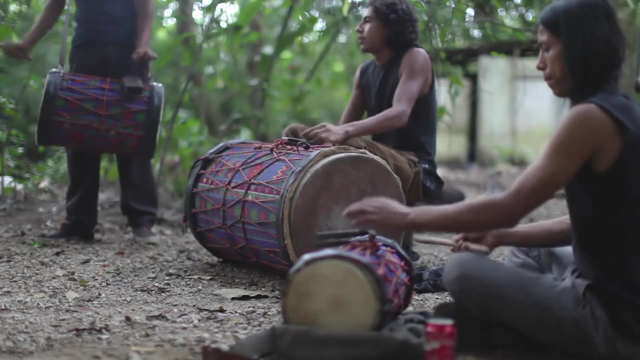 Are languages commonly spoken throughout North America. If you said English, Spanish or French, you are correct. Fun fact, Canada has two official languages, French and English. There are also many indigenous languages and dialects spoken throughout North America. Here are some noteworthy facts about the continent. 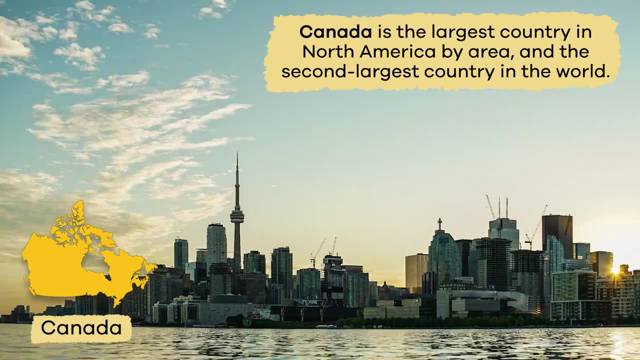 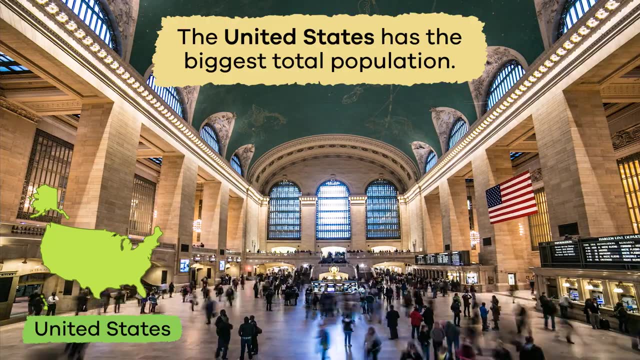 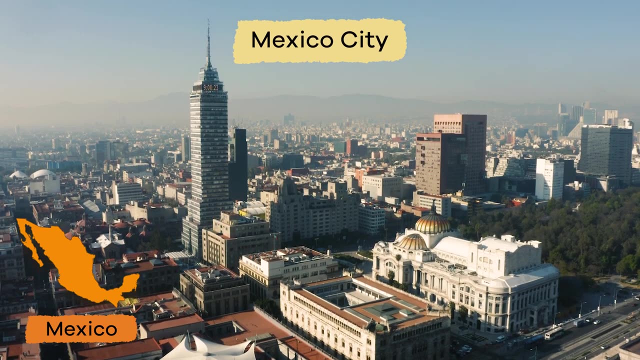 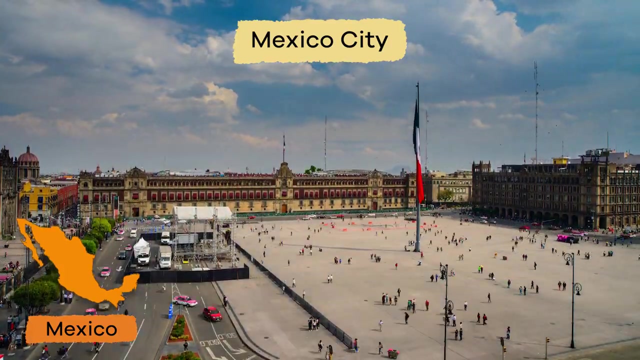 Canada is the largest country in North America by area and the second largest country in the world. The United States has the biggest total population and Mexico has the most populous city, Mexico City, with 9 million people living in the city itself, plus an additional 20 million people living in the metropolitan area outside the city. 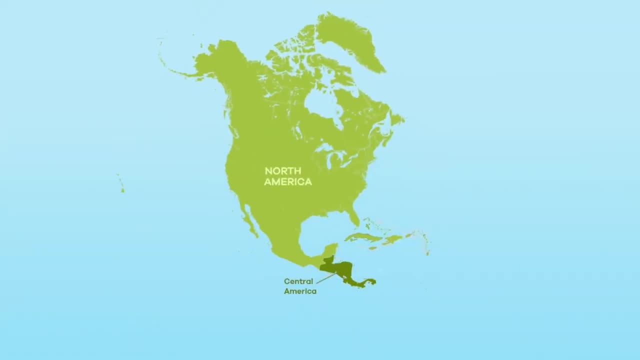 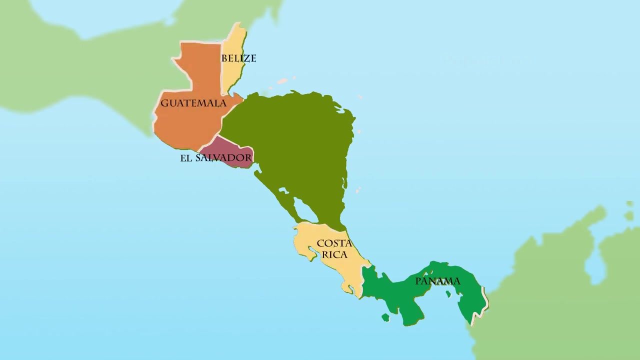 Central America is the southernmost region of the continent and connects with South America, which is another continent. There are seven countries in Central America: El Salvador, Panama, Belize, Costa Rica, Guatemala, Honduras and Nicaragua. The total population of this region. 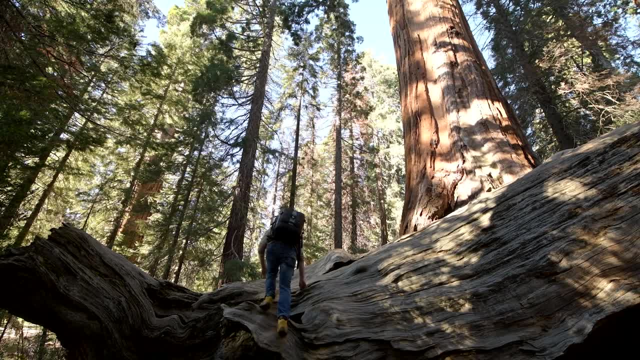 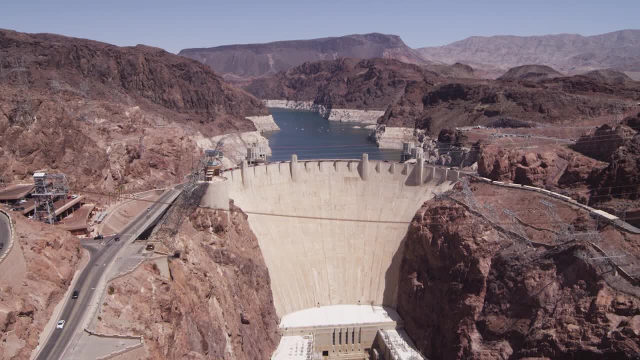 is over 50 million. There are many unique and famous attractions, both natural and man-made, all across North America. We are going to talk about 4 of them. The first one is San Francisco. The second one is San Francisco. The third one is San. 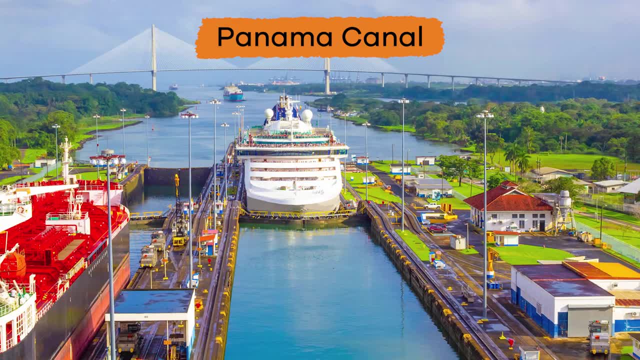 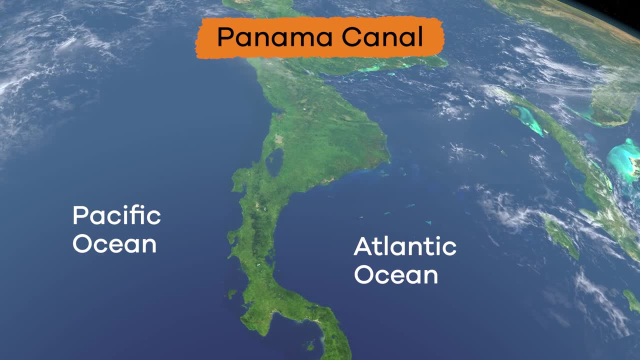 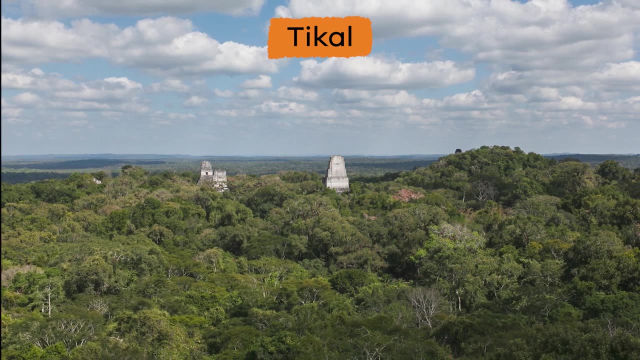 Francisco. First is the Panama Canal. It is an artificial 48-mile waterway that connects the Pacific and Atlantic Oceans and was first used in 1914.. Tikal is in a tropical rainforest in Guatemala and was an ancient Mayan city. Pyramids and temples built by the Mayans. 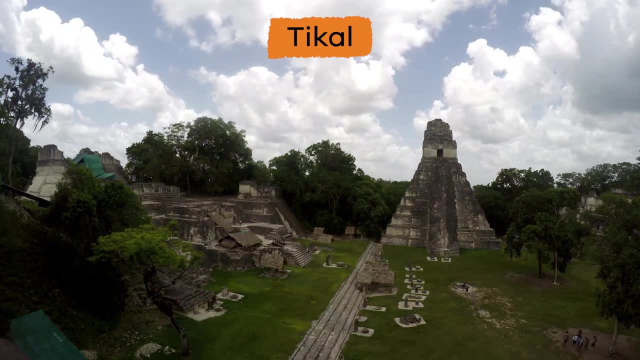 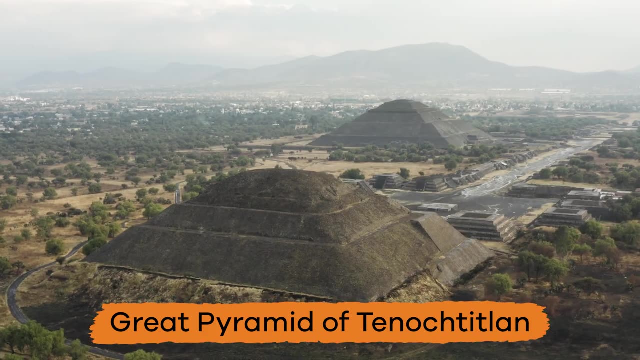 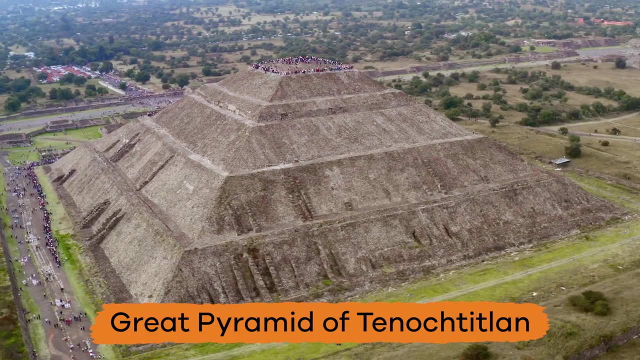 still exist there and attract many tourists. One of the main temples of the Aztecs was the Great Pyramid of Tenochtitlan, which is near present-day Mexico City. Built in the 14th century, it stands nearly 200 feet tall. Last is Niagara Falls, which is Canada's. 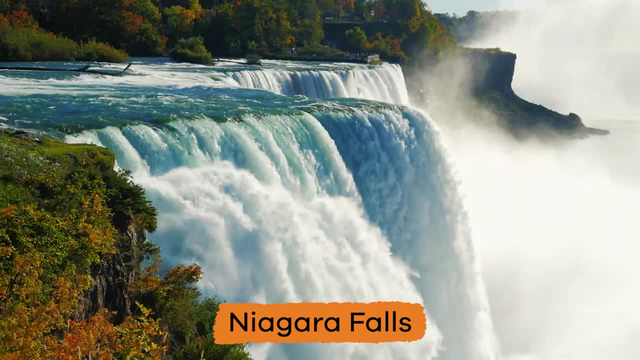 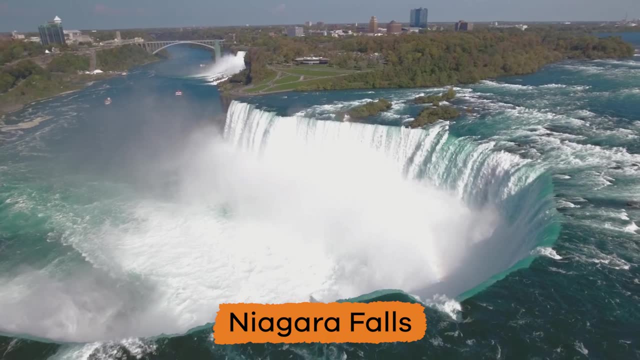 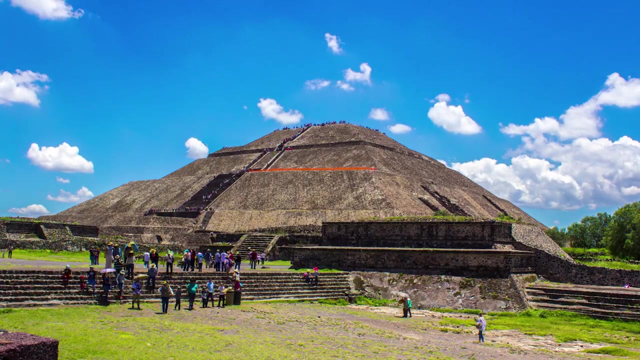 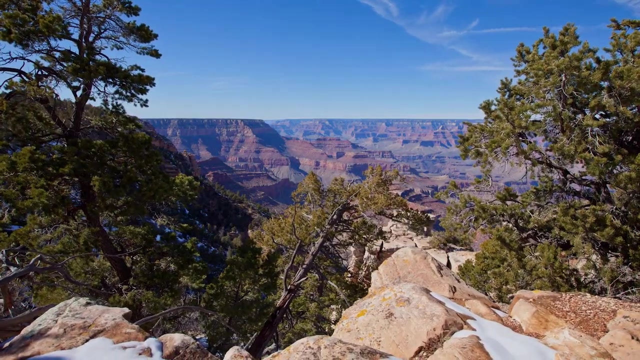 most famous natural attraction Situated on the border with the United States. Niagara Falls is 187 feet tall and has the highest flow rate of any waterfall in North America. These and many other attractions and landmarks are visited by millions of people each year. There is such a cool combination of the old and the new. 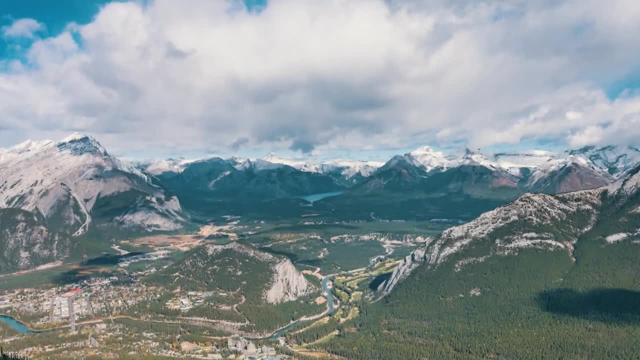 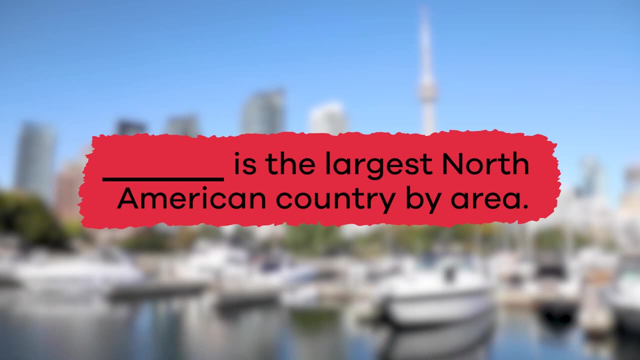 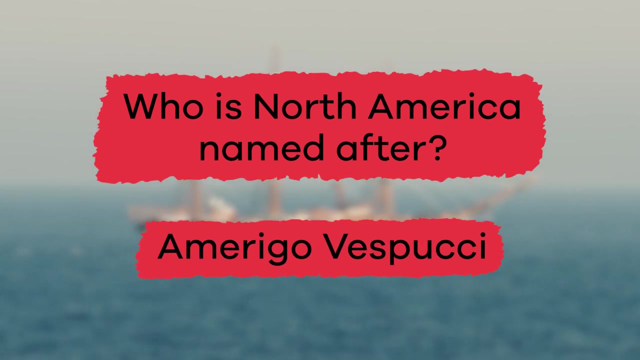 with something exciting for everybody. Now that we have learned facts about North America, let's review. Fill in the blank. Blank is the largest North American country by area: Canada. Who is North America? named after The Italian explorer, Amerigo Vespucci.